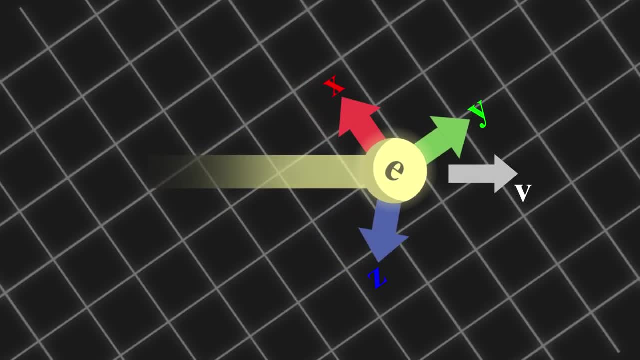 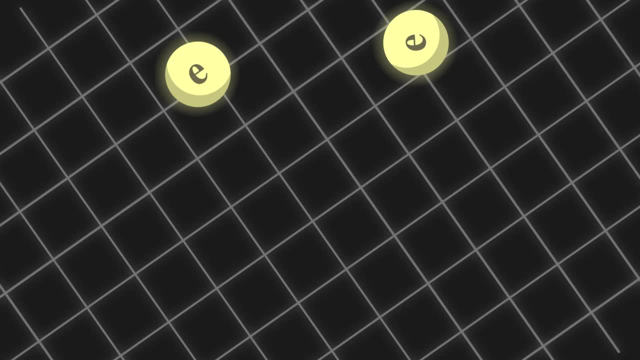 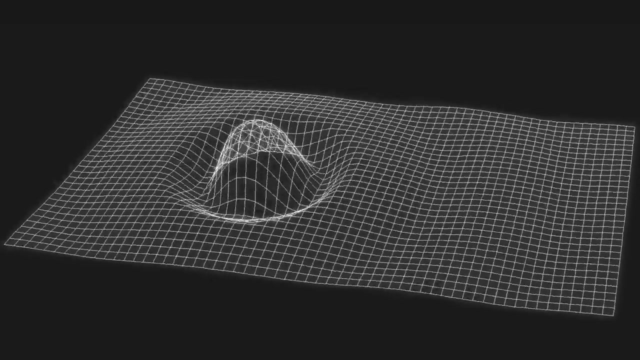 follow a certain trajectory. We know its precise position and momentum at any given point. If the particle hits one another, it will bounce off just like a ball. On the other hand, waves are not localized. They are oscillations that propagate from one place to another. You can't. 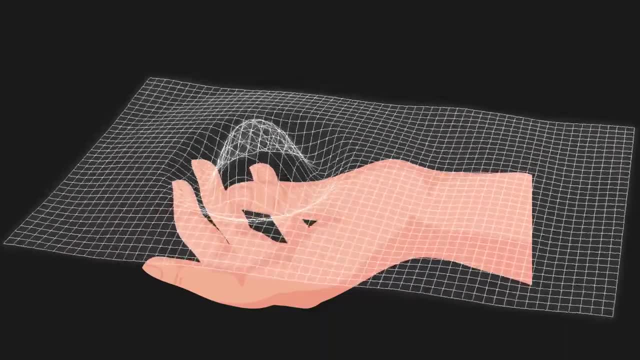 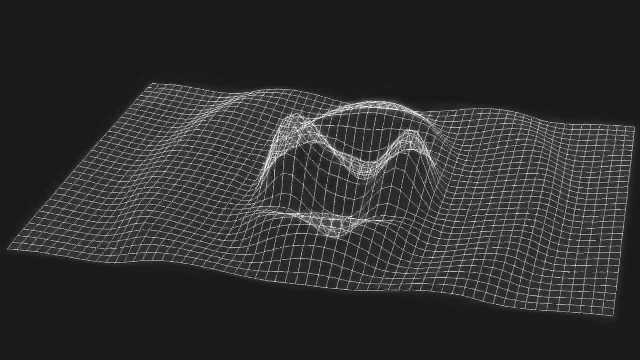 hold the wave in your hand. Instead, waves will pass over or even through your hand. When two waves come across, they interfere with each other rather than bounce off. Particles and waves are so distinct, If you want to describe something scientifically. 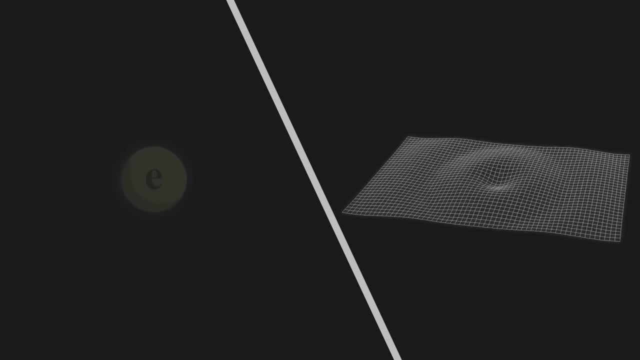 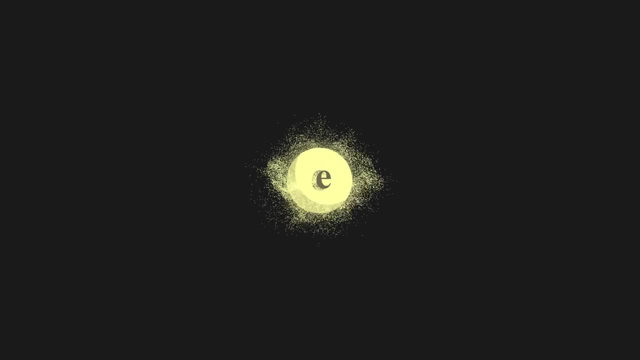 you have to be a scientist. You have to be a scientist. You have to be a scientist. You have to decide if it's a particle or wave. However, modern physics discoveries tell us all. matter exhibits both wave and particle properties, known as wave-particle duality. Electrons travel. 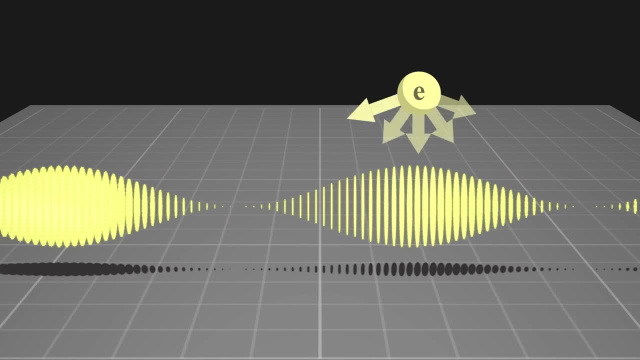 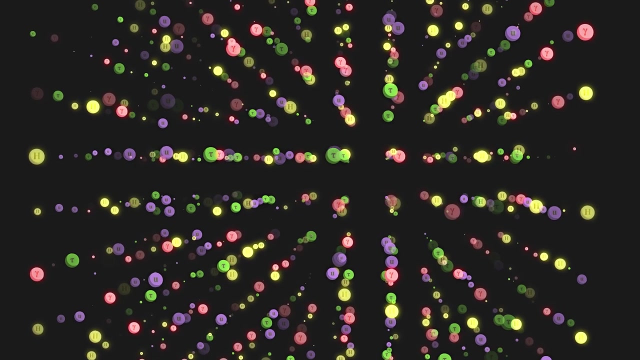 through space as wave packets. We cannot tell the exact position of the electron during its propagation, but we can predict its existence at a certain location with a specific probability which is represented by the area of each individual slice of the wave packet. Universe is the common stage for all macroscopic particles. 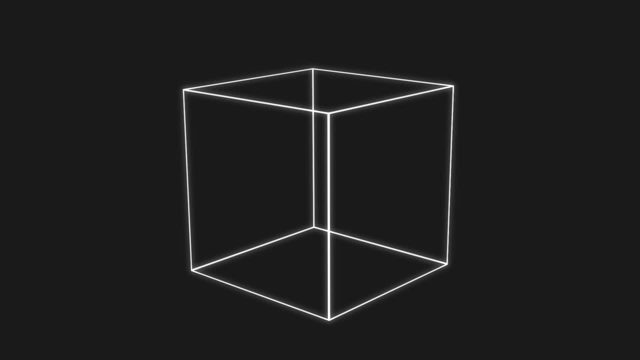 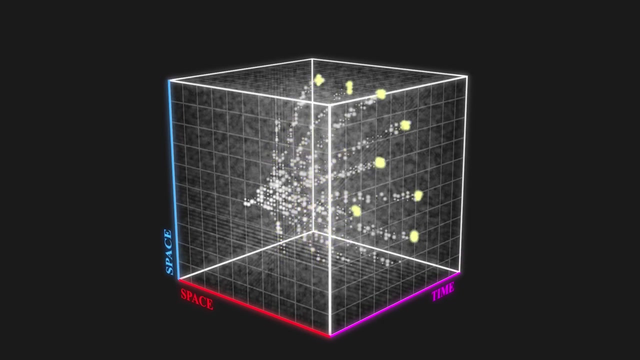 To begin with, let's start with an empty world. General relativity told us, the fabric of our universe is a 4D spacetime. To simplify, we would only represent two dimensions of space as well as one dimension of time. An electron is traveling through spacetime along an infinite. 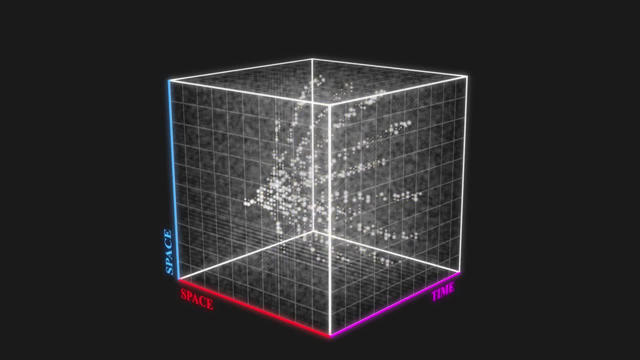 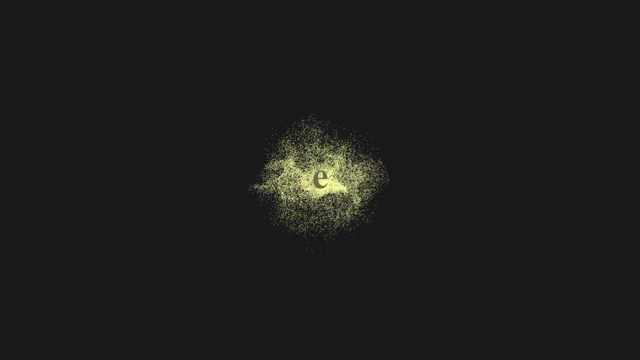 number of paths simultaneously. Each path has a different probability to be selected by the electron. However, when the electron reaches the screen, it will suddenly collapse into a particle and only hit in one place with specific momentum. Sometimes the electron acts like a wave, Sometimes 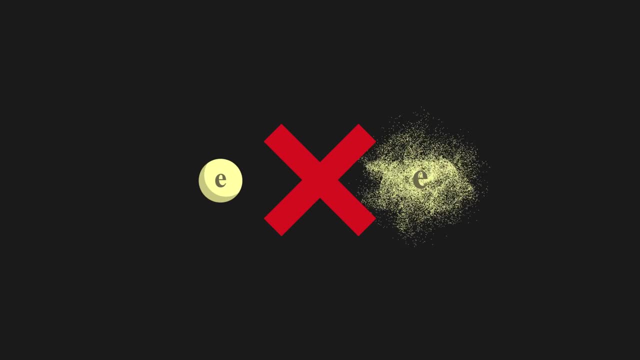 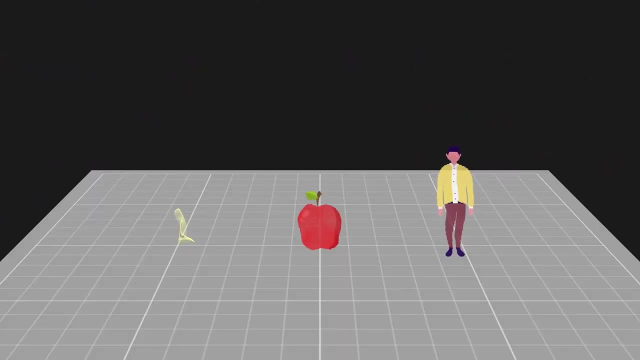 it acts like a particle, but never both at the same time. Wave-particle duality is not confined to macroscopic particles. Instead, everything exhibits wave-particle duality. However, as objects get larger, they are associated with a different probability. For example, if a particle is 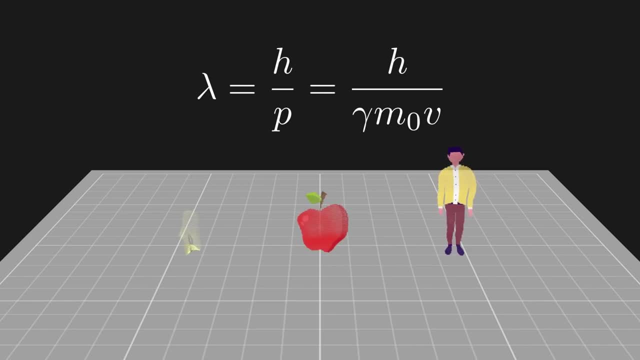 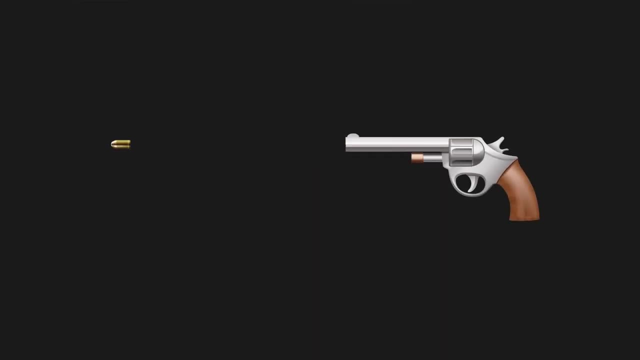 larger. its wave-particle duality is neglected in the macro world. That is why, if you shoot a bullet, only one person will be killed at a time. Thanks for watching. If you like my video, please subscribe to this channel.